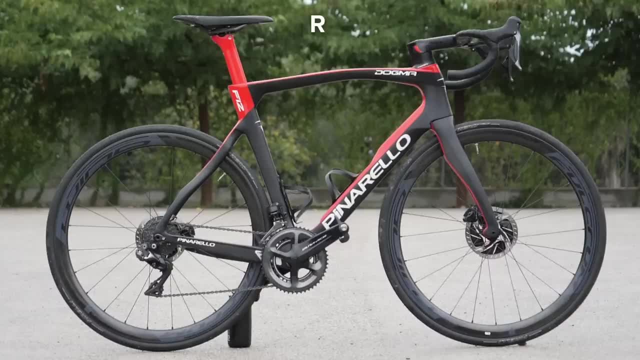 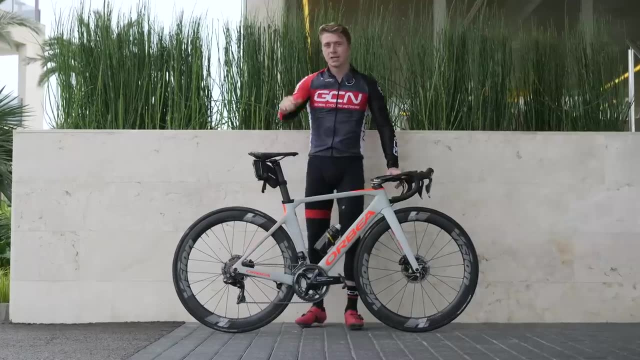 also come with a leg length. Much like buying trousers, you will have to try on several pairs or ride several different bikes to find the perfect fit for you. Before we get onto that, though, let's get one easy, but fundamental point under our belts. 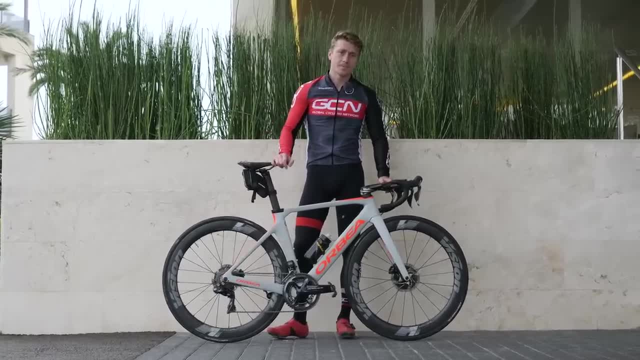 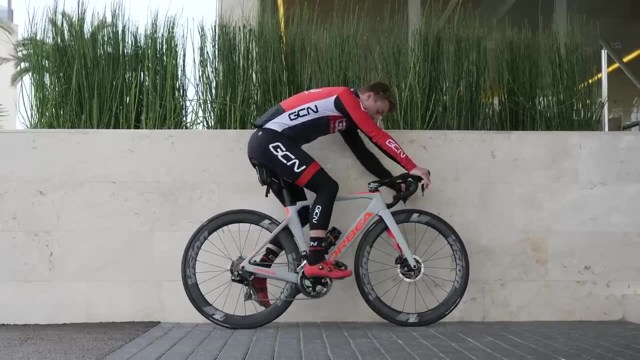 first, That is, what is our saddle height and how can we find it? A really easy way is to find a wall like this: get onto your bike placing both hands on the handlebars. place one pedal all the way down to 6 o'clock Now. put your heel on the pedal Now. 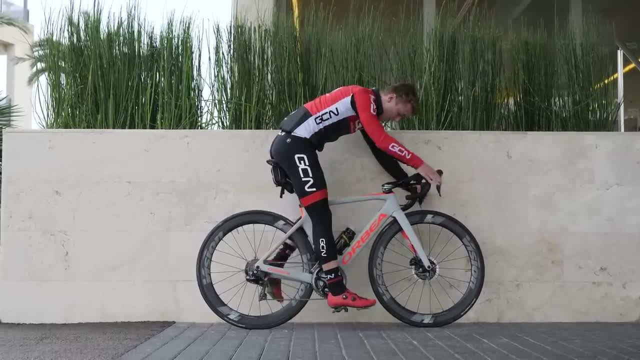 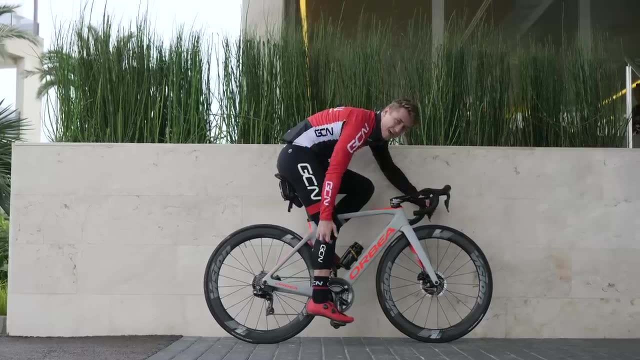 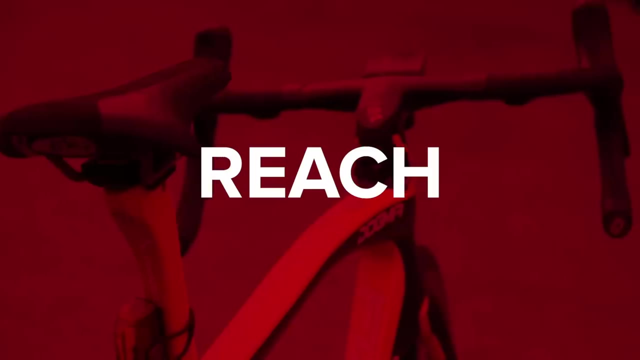 you should find your leg straight. Then when you go to clip in and put it back into normal position, you find your leg is slightly bent. Really easy but really effective way of finding the right saddle height for you. Finding your correct saddle height is: 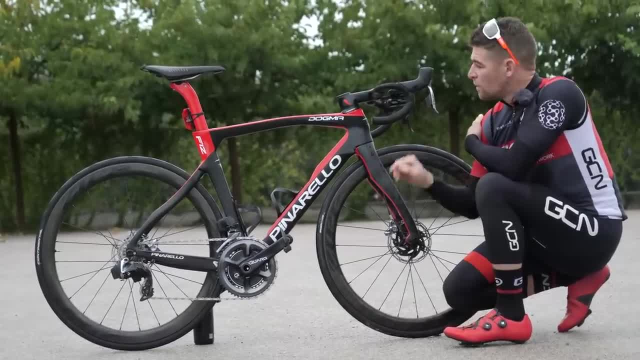 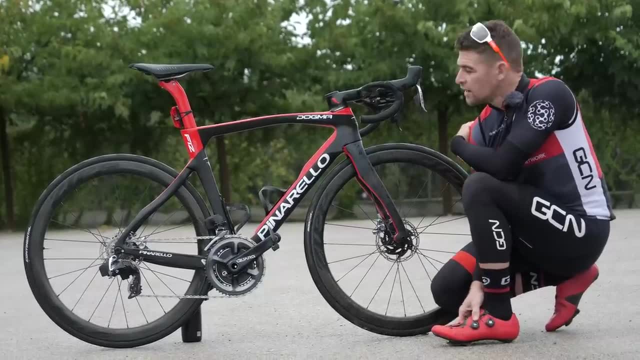 relatively easy, and that's because you've got plenty of scope for adjustment. When it comes to setting your reach, though, you're much more restricted in the adjustments that you can make, even though it is potentially more important to your comfort on the bike- The reach of different. 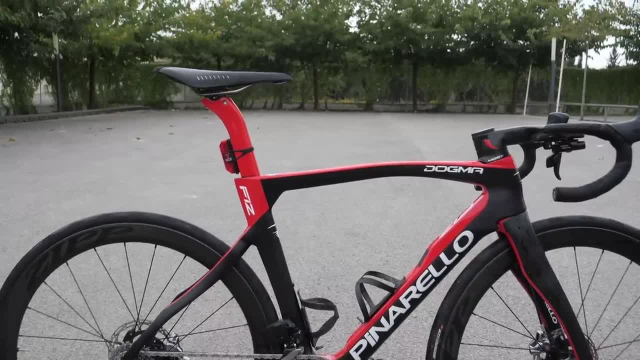 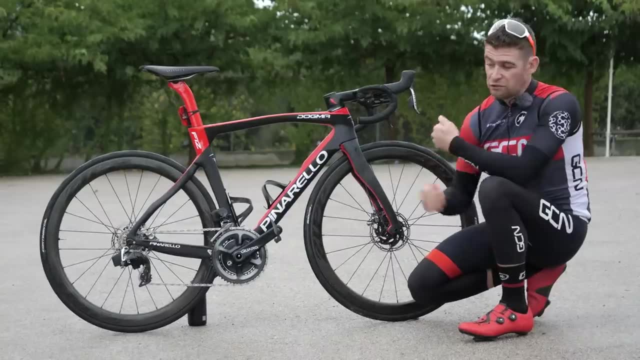 bikes will vary within a manufacturer, but also from brand to brand. This depends on the type of riding the bike is designed for, but also the size of the bike you're riding. Racing bikes, like the ones you'll see at the Tour de France, is generally really long and really low, whereas a gravel bike 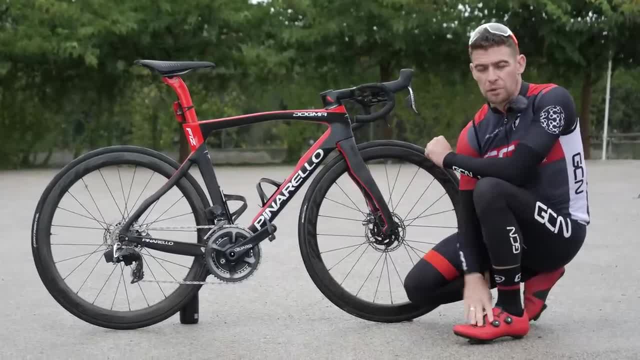 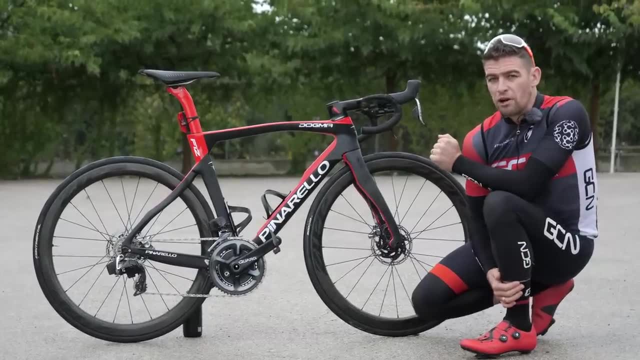 will be a little bit shorter and higher. The numbers that refer to how the bike will be are known as stack and reach, if you remember those from earlier. If you're new to cycling, relatively more relaxed about your riding, or you're a little bit less flexible, you'll probably 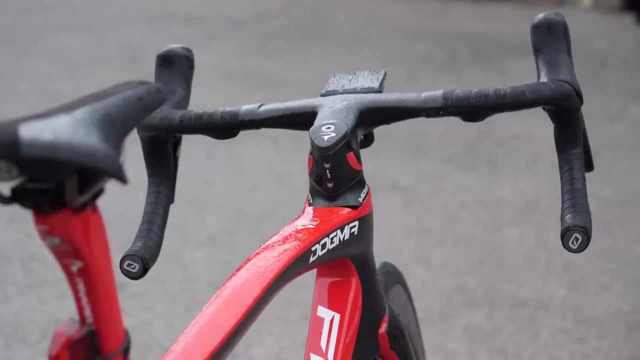 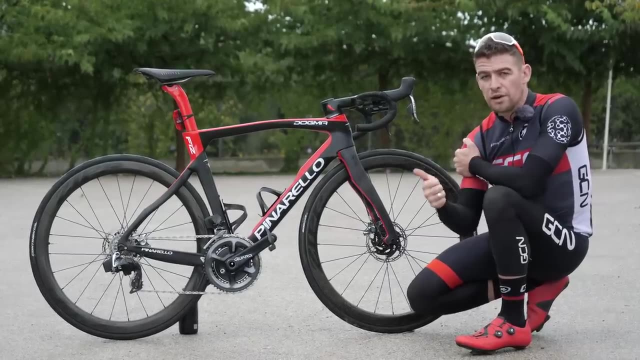 favor something that's shorter and higher, Whereas if you're into racing, you'll probably favor something that's longer and lower. For example, of different types of geometry. Canyon put their three bikes into different categories: pro, pro sport and sport geometry. How will you decide? 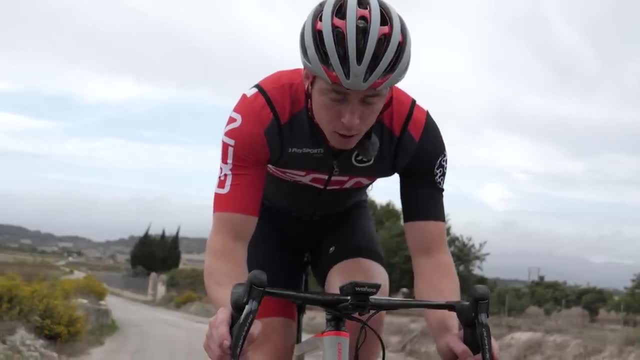 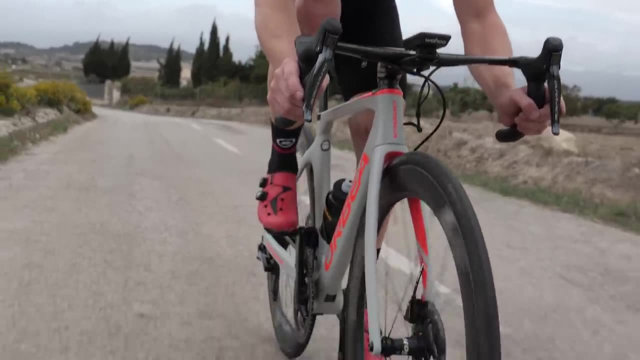 on where your bars need to go. This is going to depend on a few things. If you have long arms, a long back and you're very flexible, you'll probably be able to get yourself into a longer lower position. If you're less flexible or you have a shorter back and arms, then the opposite. 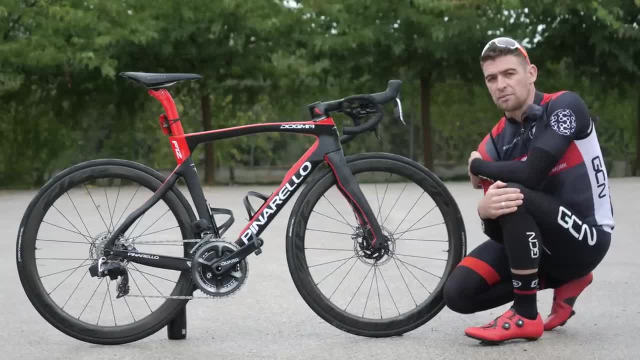 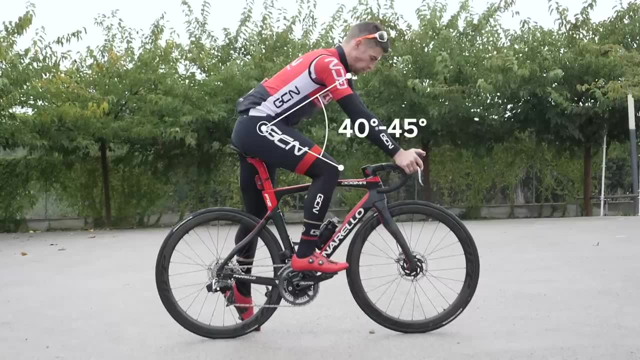 is, of course, true as well. Then, finally, the type of riding that you do is going to play a factor as well. Generally speaking, though, with your saddle in the correct position, the relationship from your shoulder to hip angle should be 40 to 45 degrees to horizontal.